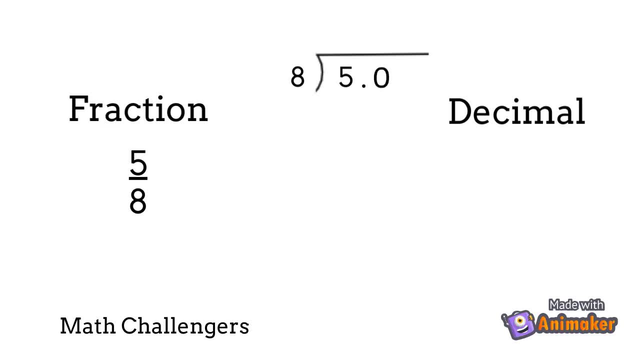 To do that we have to add decimal point in the dividend and 0. if needed, Put the decimal point in the quotient directly above the decimal point in the dividend. Then divide like whole number. Just write in decimal afterwards. much as you would do with what you use. 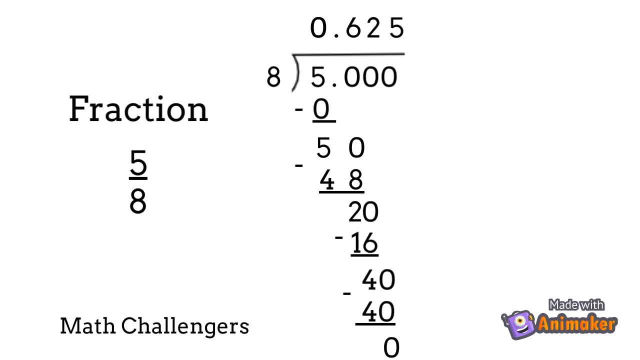 Let's do the same for half- Tre Kosh-Tek. The fraction 5 eighths is equal to six hundred twenty five thousandths in decimal. If we have cubed it within the indicator, we can express our score to a decimal. 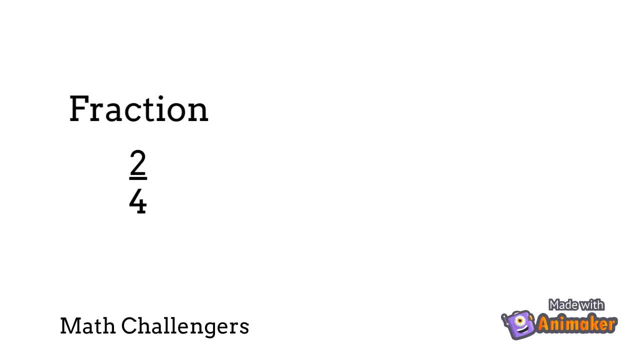 It can also be expressed as a decimal. if we want a number to be a decimal, We can also worry aboutред speaks words accurately. 2. fourth is 5 tenths in decimal. In case of a mixed number, just divide the numerator by the denominator. 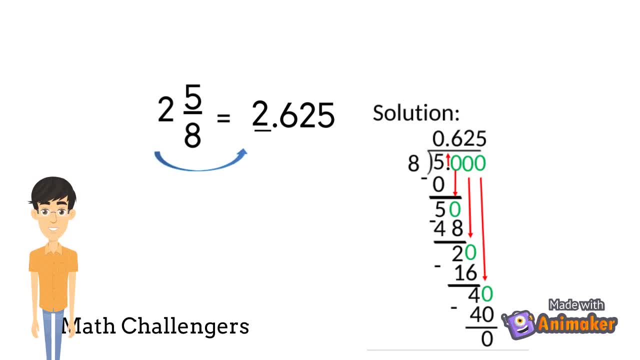 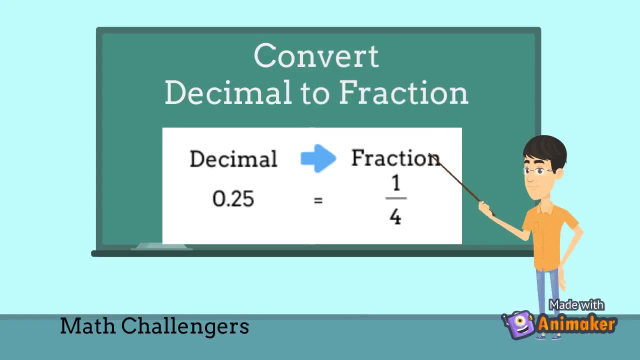 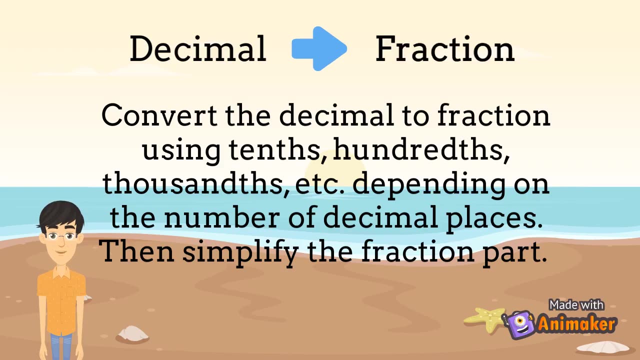 And the whole number is written on the left side of the decimal point. 2 and 5 eighths is 2 and 625 thousandths. Convert decimal to fraction. Convert the decimal to fraction using tenths, hundredths, thousandths, etc. depending on. 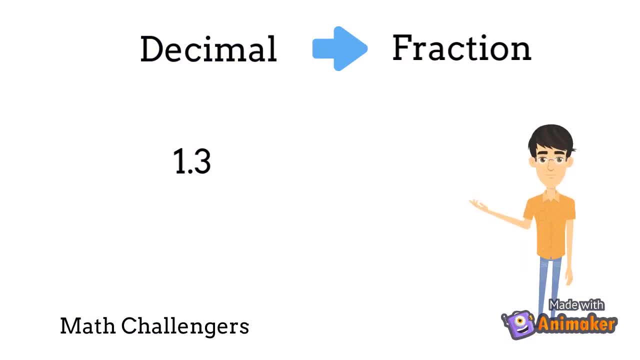 the number of decimal places. Then simplify the fraction part To change 1 and 3 tenths to fraction. The digits on the left side of the decimal point is the whole number And the digits on the right of the decimal point becomes the numerator. 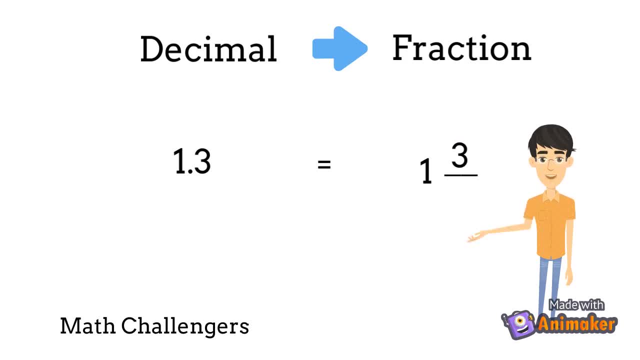 The denominator will depend on the number of decimal places. If the number has 1 decimal place, then the denominator is 10,. if it has 2 decimal places, then the denominator is 100.. If 3,, the denominator is 1000.. 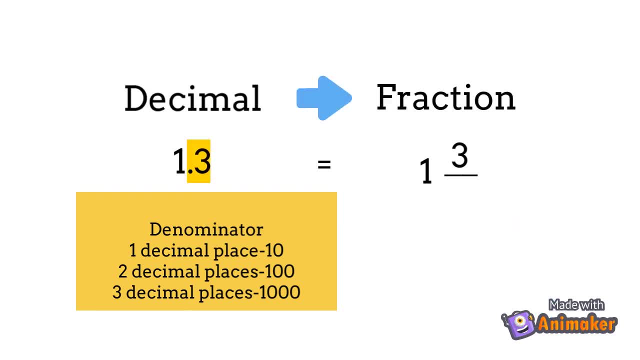 When we say decimal places, We mean the number of digits on the right side of the decimal point. In this case, we only have 1 decimal place. Therefore, the denominator is 10.. Make sure to reduce the fraction part to its lowest term. 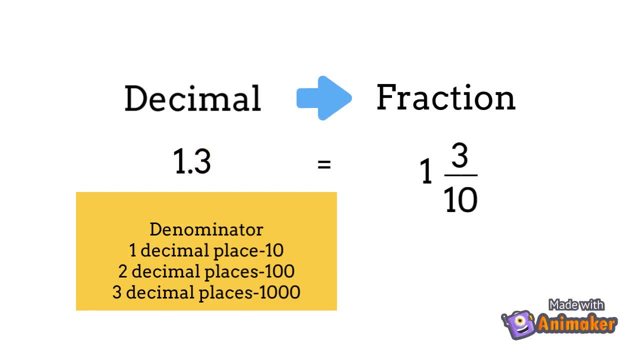 If possible To change. 25 hundredths is fraction. The digit on the left of the decimal point is 0, so there is no whole number. The digits on the right of the decimal point, Which is 25, becomes the numerator And the denominator is 1.. 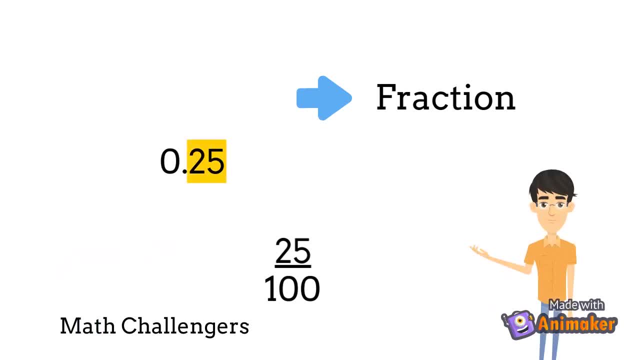 And the denominator is 1.. And the denominator is 100 because we have 2 decimal places. Since the 25 hundredths is not yet in its lowest term, Then we can divide both numerator and denominator by their GCF, which is 25.. 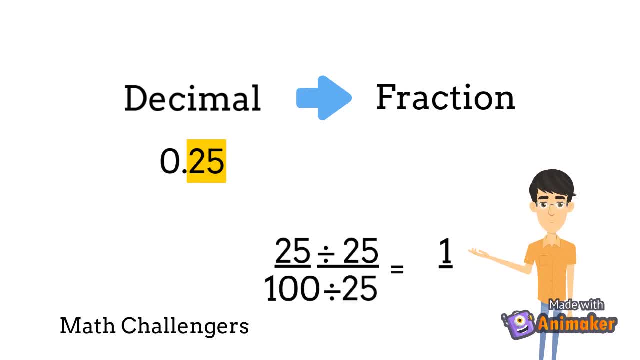 So 25 divided by 25 is 1.. And 100 divided by 25 is 4.. 25 hundredths in fraction is 1. fourth, Let's do another one: What is 3 and 15 thousandths in fraction? 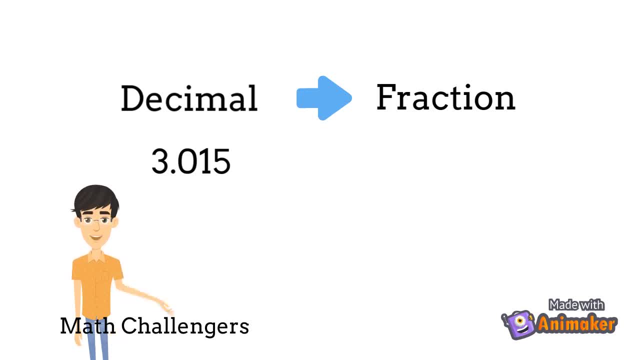 What is 3 and 15 thousandths in fraction? The digit in the left side of the decimal point is the whole number. The digit in the left side of the decimal point is the whole number. The digit in the left side of the decimal point is the whole number. 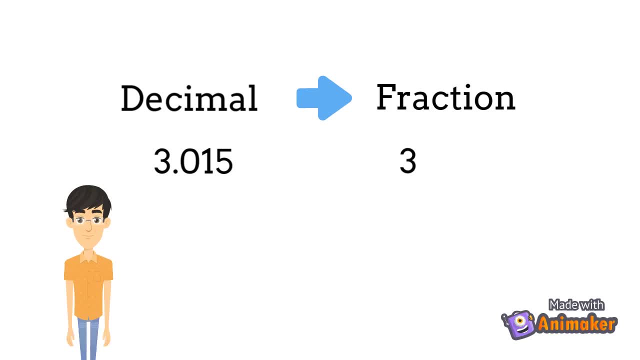 The digits on the right side of the decimal point is the fraction part. The digits on the right side of the decimal point is the fraction part. 15 becomes the numerator, and since there are 3 digits on the right of the decimal point, Then the denominator is 1000.. 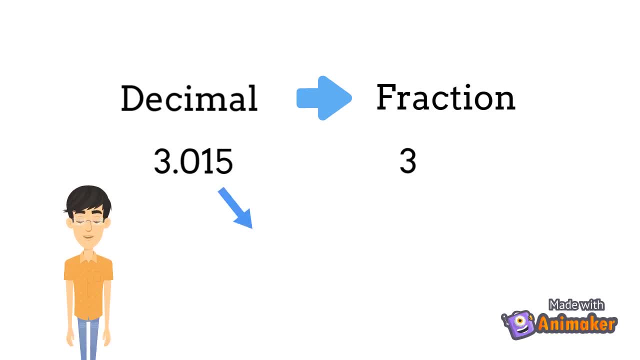 Then the denominator is 1000. But notice that 15 thousandths can still be reduced to its lowest term, since both are divisible by 5.. But notice that 15 thousandths can still be reduced to its lowest term, since both are. 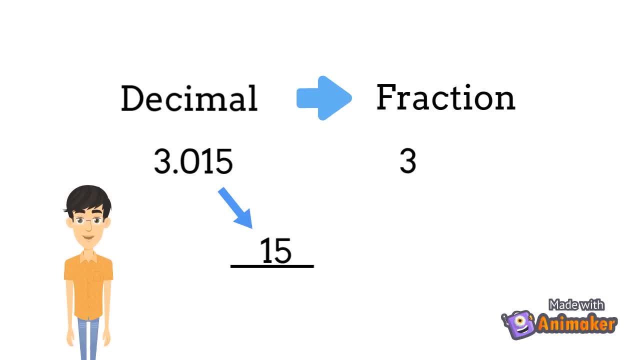 divisible by 5.. But notice that 15 thousandths can still be reduced to its lowest term, since both are becomes the numerator, and since there are three digits on the right of the decimal point, then the denominator is 1000.. But notice that 15 thousandths can still be reduced to its lowest term, since both are. 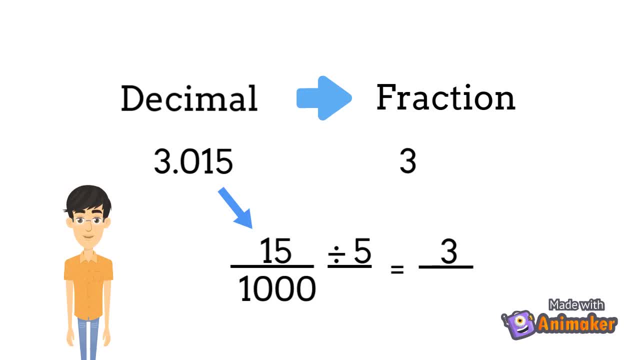 divisible by 5.. 15 divided by 5 is 3 and 1000 divided by 5 is 200. Therefore, the fraction form of 3 and 15 thousandths, in lowest term, is 3 and 3 over 200.. 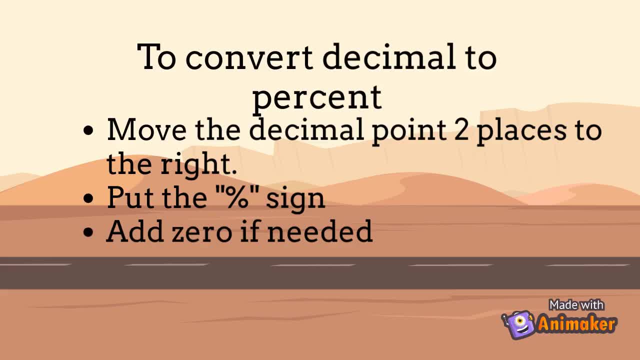 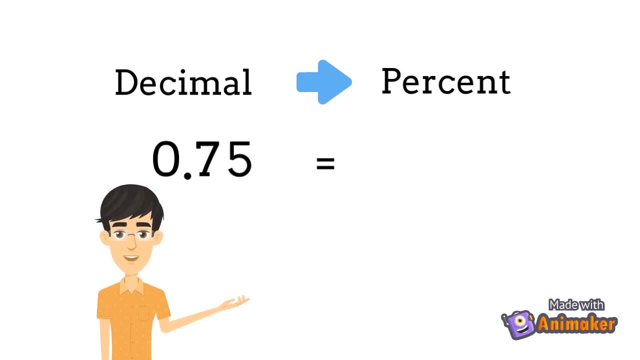 Now let's have changing decimal to percent. To change decimal to percent, first move the decimal point two places to the right, then put the percent sign. Add 0 if needed. Example: change 75 hundredths to percent. To do that we have to move the decimal point two places to the right, then put the percent. 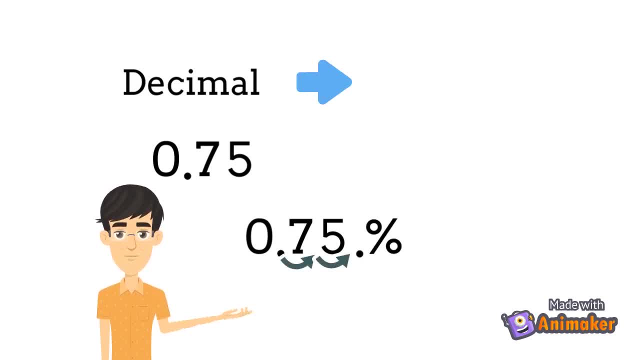 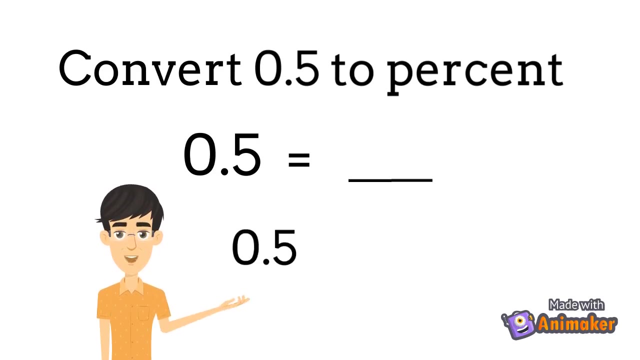 symbol. The decimal 75 hundredths in percent is 75.. Let's convert five-tenths to percent. Again, to convert decimal to percent, just move the decimal point two places to the right. then put the percent symbol. Add 0 if needed. 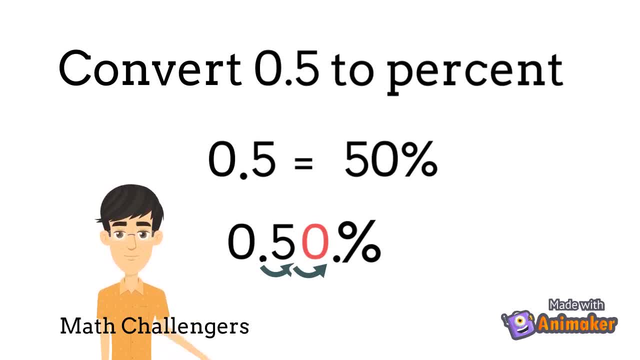 Five-tenths to percent is 50 percent. To convert decimal to percent, just move the decimal point two places to the right. then put the percent symbol. To convert decimal to percent, just move the decimal point two places to the right then. 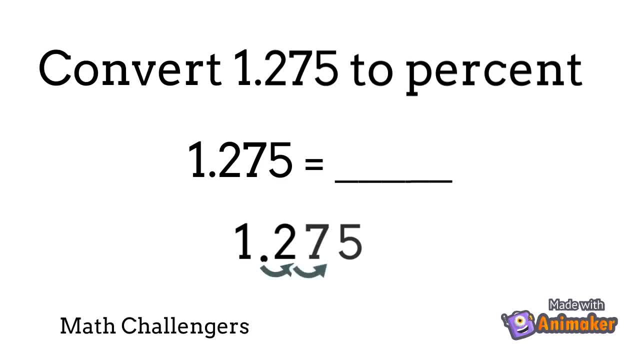 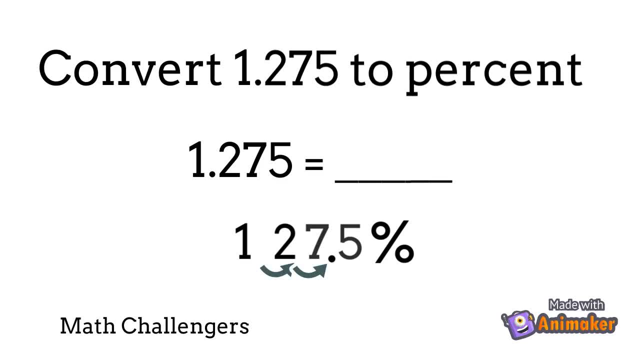 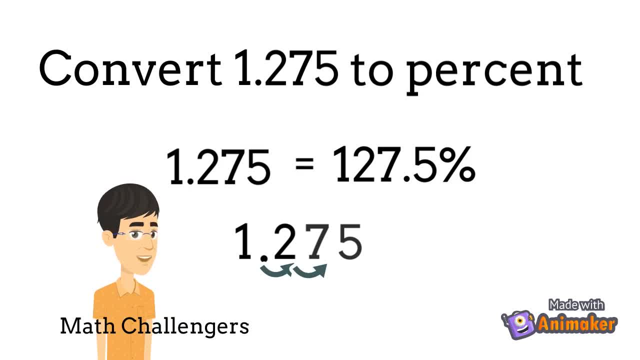 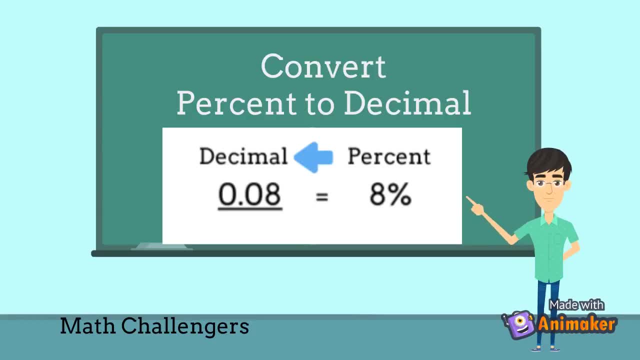 then put the percent symbol Again. to convert decimal to percent, just move the decimal point two places to the right. 1 and 275 thousandths in percent is 127.5 percent. Let us now learn how to convert percent to decimal. 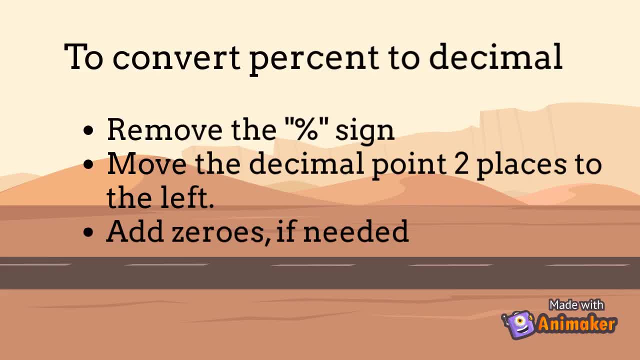 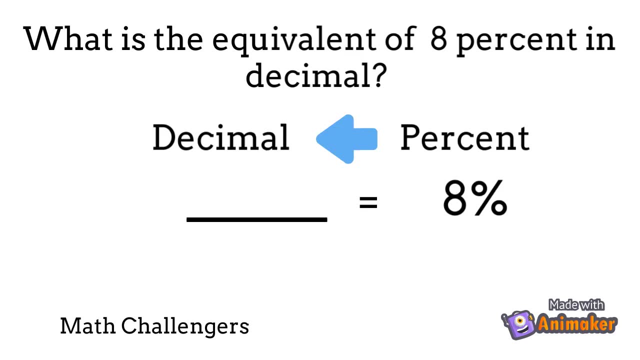 To convert percent back to decimal: remove the percent sign. Move the decimal point two places to the left. Add zeros if needed. For example, what is 8 percent in decimal? First remove the percent sign. Then move the decimal point two places to the left. 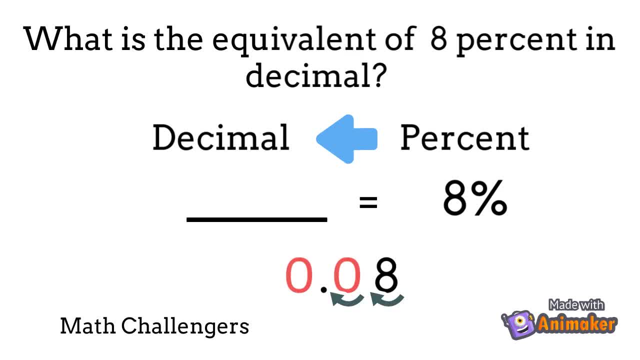 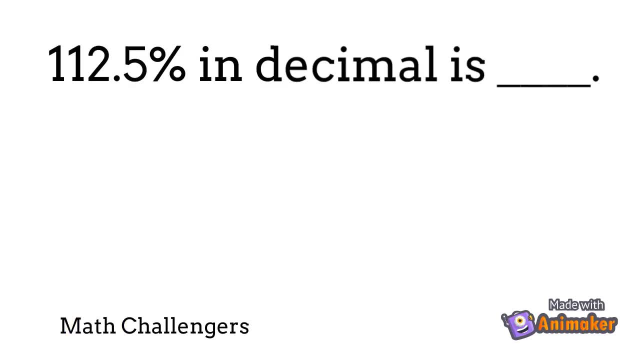 Add zeros if needed. 8 percent in decimal is eight hundredths. Another example of converting percent to decimal: Change 112.5 percent to decimal. Again, remove the percent symbol. Then move the decimal point two places to the left And you can add zeros if needed. 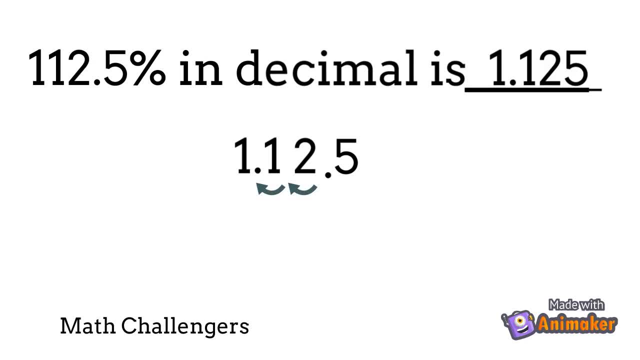 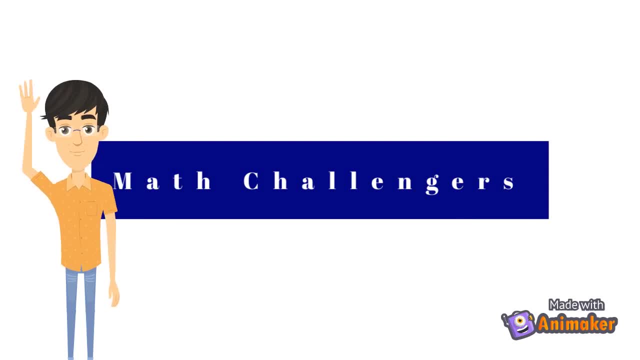 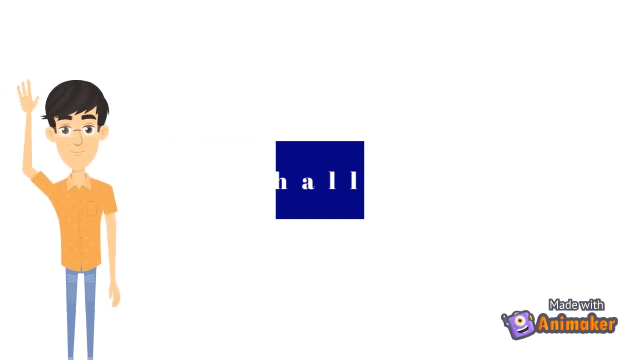 112.5 percent is 1 and 125 thousandths in decimal. Thanks for watching. Drop a like, Leave a comment And don't forget to subscribe. See you in the next video.